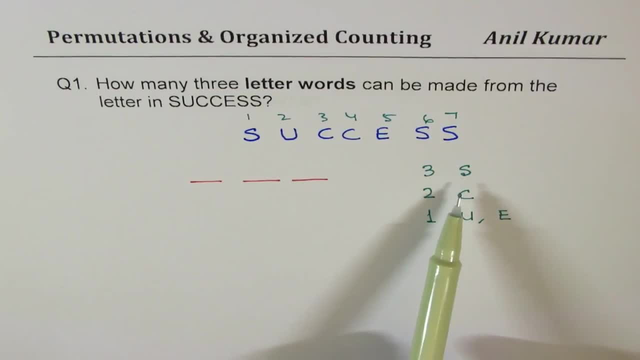 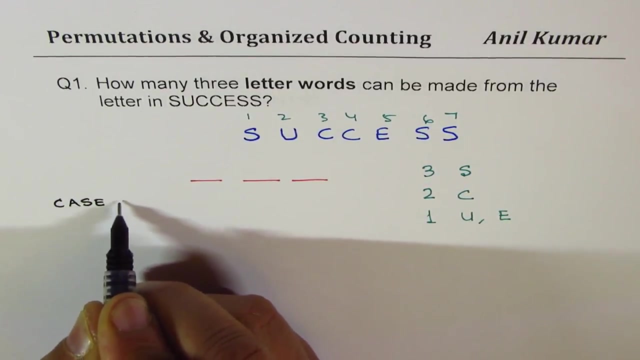 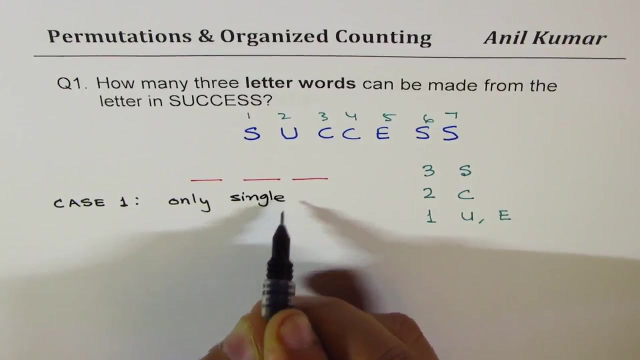 Now, since you can see, some letters can come twice, some can even come three times. So in this case we should actually go with cases. So let's see how to organize our cases. So let's say case 1. Here we will take only single letters, no repetition. 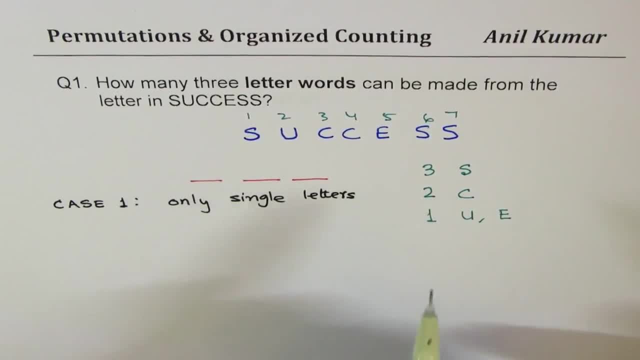 When I say only single letters, that means we will be working with only one S, only one C, only one U and one E. You get the idea right. So so we are working only with four letters And we have to focus on one letter. 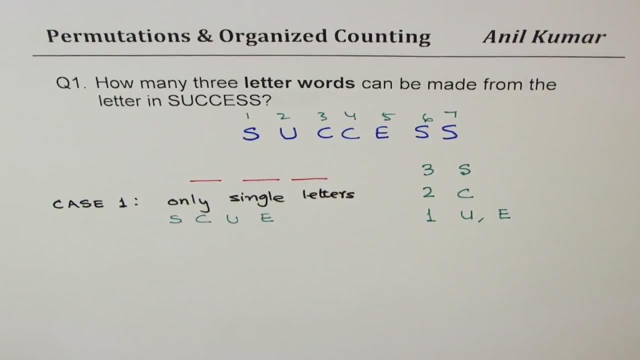 And we have to fill in five spaces. Nothing is repeated. So how many ways can you do it? Well, we are doing four Out of four, we are selecting three. So 4P3 is the answer correct. So that is case 1.. 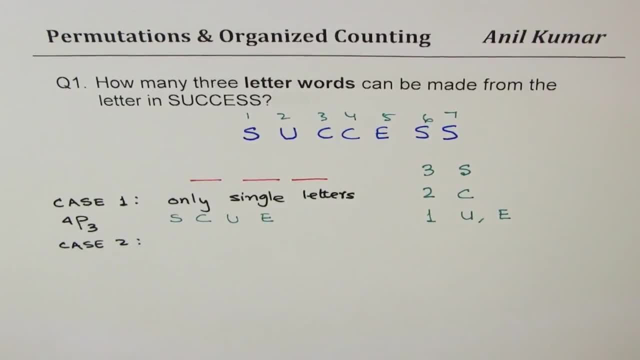 Now let's do case 2.. In case 2, we will take one double. That means one letter will be repeated, right? So only one double, right, One double only. Let me write like this: So in that case we have two possibilities. 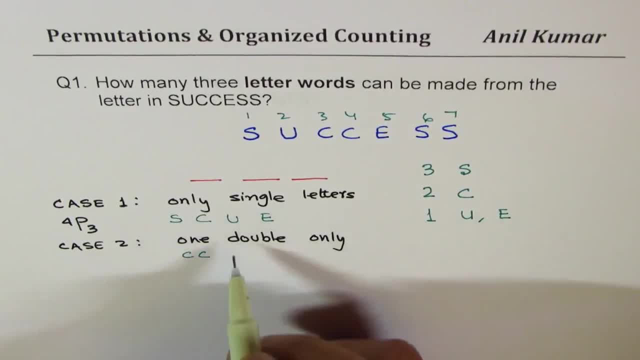 We could have two C's along with the, along with any of the others which are S, U and E, right, Or we could have two S With C, U or E, correct? So that becomes next combination, Okay. 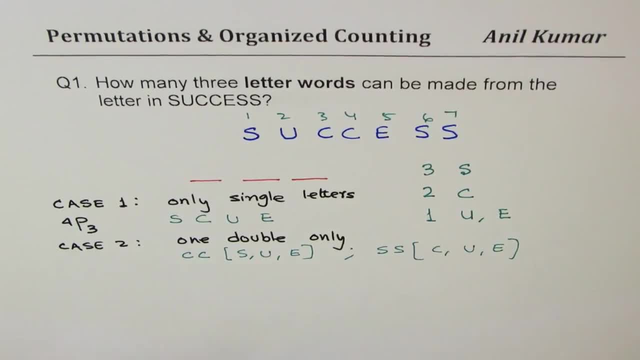 So let's look into this one first. So again, we are left with three spaces. So we are going to fill these three spaces with two C's first. Now, how many ways can we do that? Well, two C's means there's a repetition. 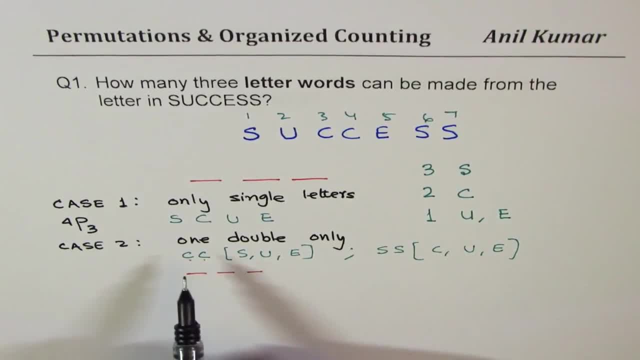 But we are filling these spaces and total number of letters, total number of places, are three. Two C's to be filled, So that becomes 3P2,, correct, 3P2.. Two C's can be filled in Now. once you fill in two C's, then one of these three can get into. 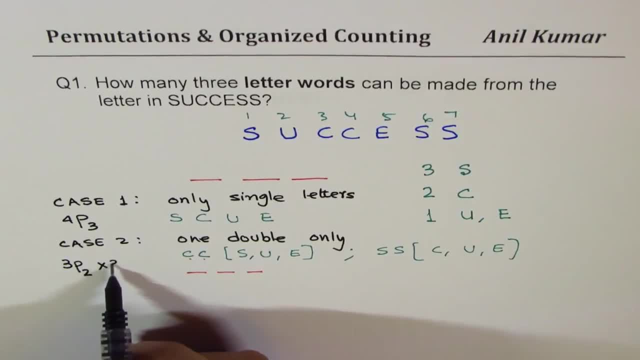 So those are three different ways. So I'll multiply that by three, And now we could have double with S also. So times two. Does it make sense to you? Correct? So you get the idea. First, we'll fill up these two C's. 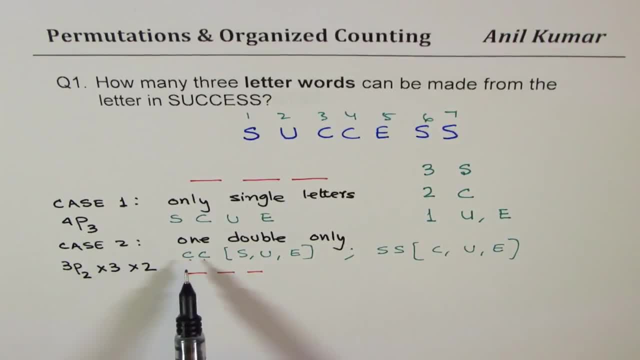 We have 2P2.. Now I forgot to write Divided by two factorials. Since they are not a C here and C there and they are reversed, we'll just give me one combination. So we have to divide by two factorial. 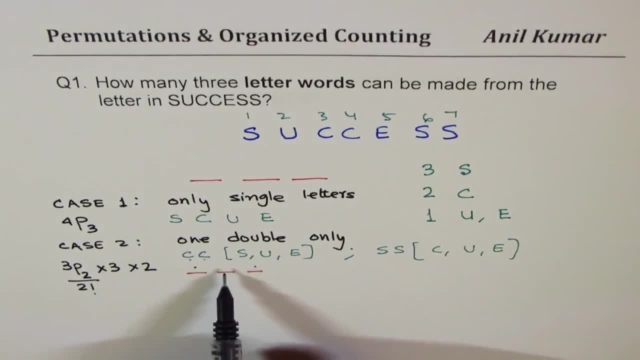 Got it right, Then three of these letters can come one by one. So times three. So we get with two C's. Now same story is to be repeated with two S. So that's what you get, Is it okay? 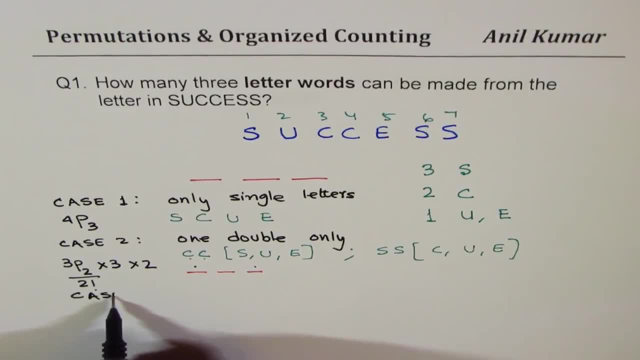 Now let's talk about case three. So in case three we have triple, Because we cannot have two doubles right. We are only limited with three positions, So we can have a triple. Triple combination is only one right, So which is only one for us. 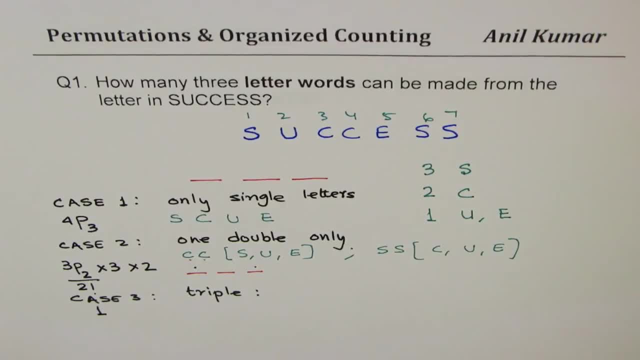 Is it okay? Now, combining all, we get our final answer right. So we can combine all this. So we get our answer as total of all this, which is 4P3 plus 3P2 divided by two factorial times, three times two plus one. 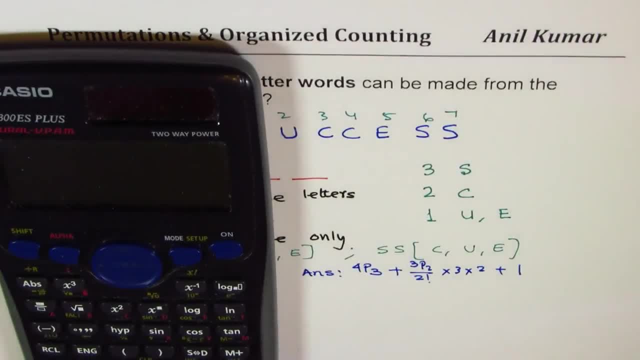 You get an idea right, Let's calculate and write down the answer. So we have 4P3, which is 24, plus 3P2 equals two. So two factorial and two factorial gets cancelled. We'll just multiply six by three.